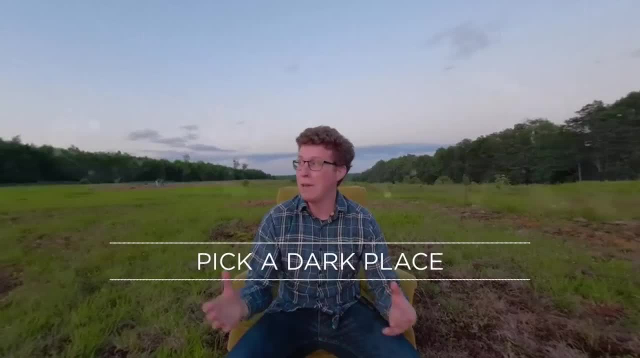 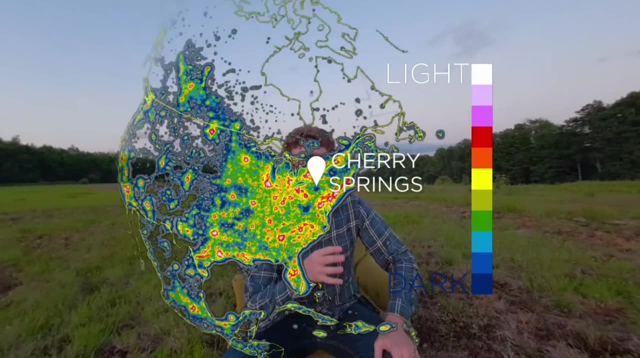 The first tip is to get as far away from city lights as possible. I'm here in northern Pennsylvania, in Cherry Springs State Park, And if you look at this map of light pollution, you can see that this is an area that's one of the darkest patches east of the Mississippi. 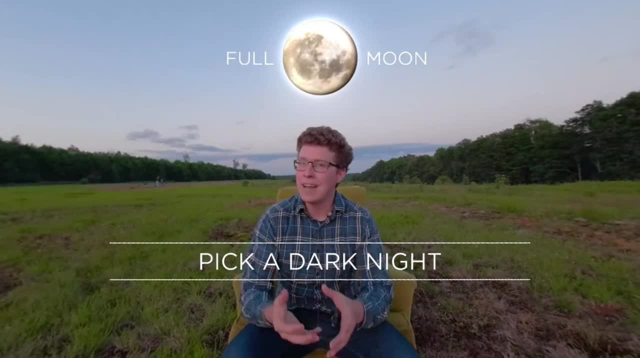 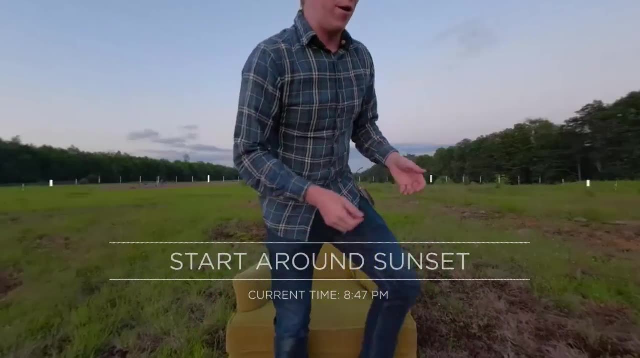 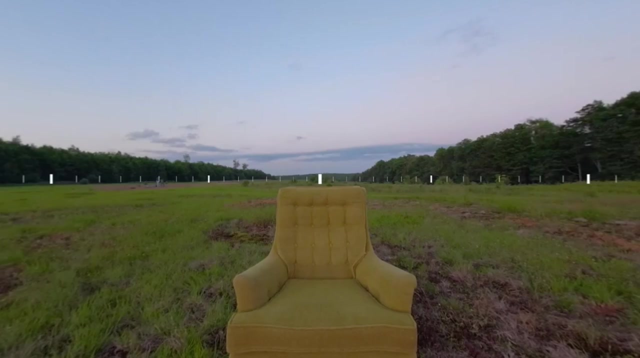 You also want to avoid moonlight and luckily tonight the moon will be just a sliver. If you start your stargazing trip around sunset, you can start to get your bearings, And this is a 360 degree video so you can look around by moving your device or by clicking and dragging. 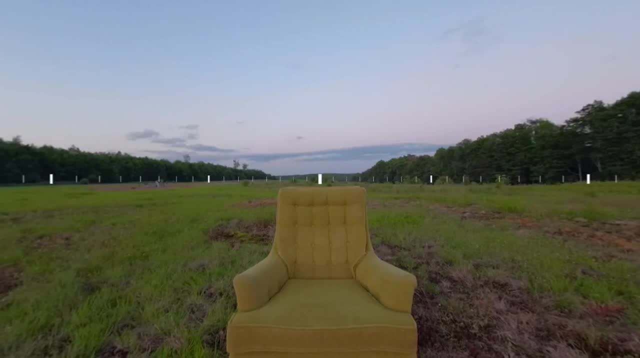 The sun just set behind me, and so that's the west. This way is north, there's south and back by the chair is east. If you look around, you'll start to see a few points of light. Some are the brightest stars and some are planets, a term that comes from the ancient Greek word for 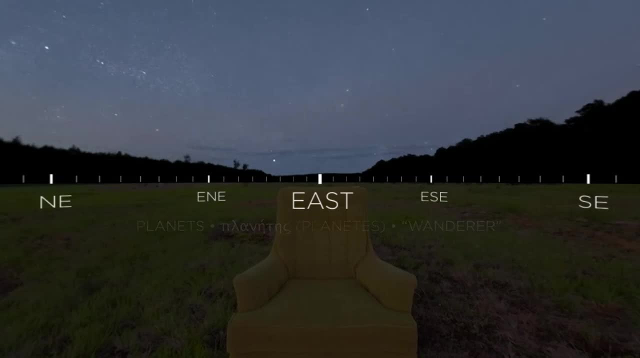 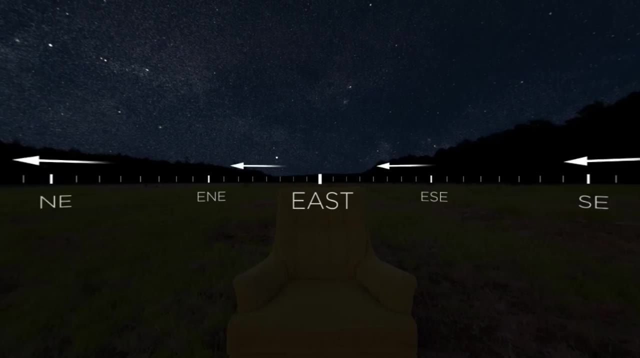 ponderer. They don't stay in the same place but rove across the fixed pattern of the stars As night falls. turn to the north and look up. Just follow these arrows and we'll start our tour. You might recognize one group of stars: the Big Dipper. 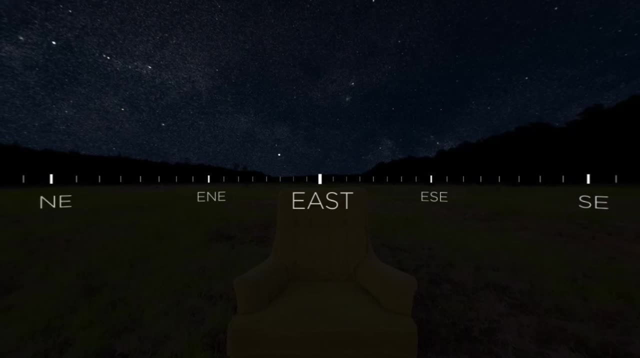 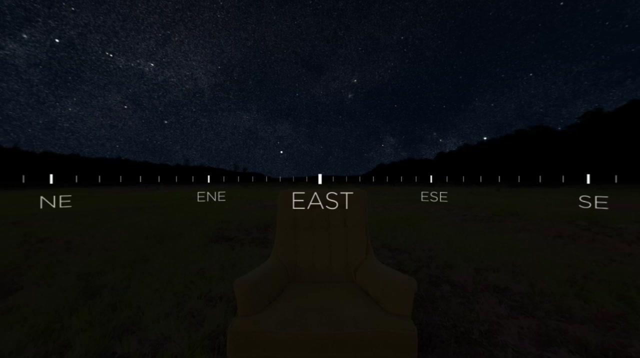 Four stars form the bowl and three more the handle. Before optometry, some tested their vision by finding an extra star in the handle, little alcor. This pair is called the horse and rider. The Big Dipper isn't an official constellation. it's technically part of Ursa Major. 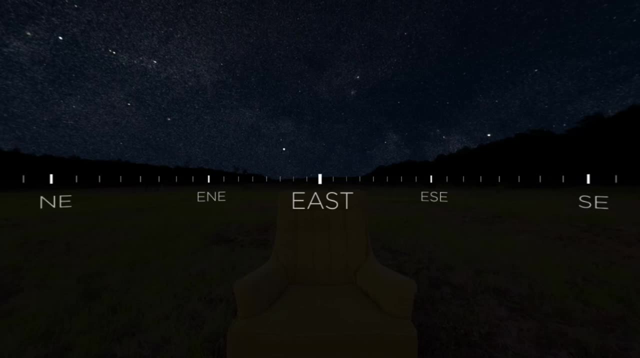 According to myth, Zeus was the king of Ursa. Major Zeus stretched out this great bear's tail as he flung it into the heavens. In Greek, bear is arktos and the lands that lay in the direction of this bear north. 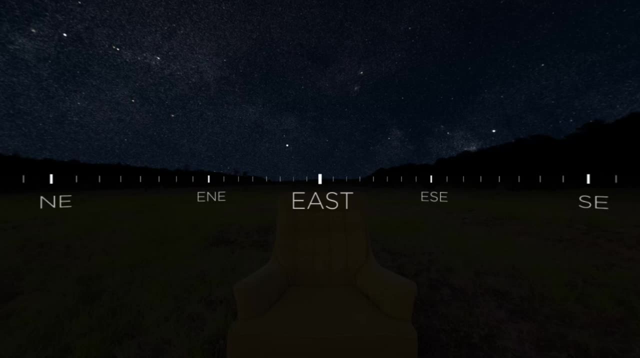 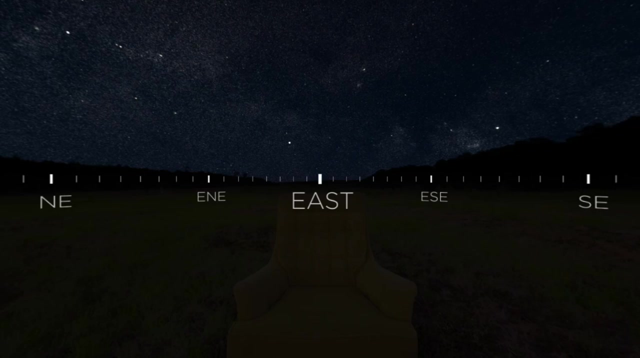 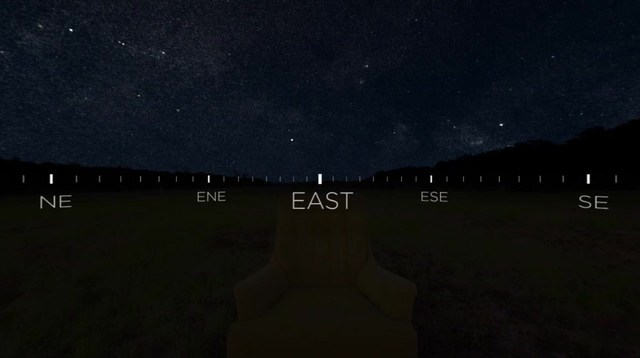 became known as the Arctic. Some Native Americans also saw a bear in these stars, pursued by hunters. In South Korea, they saw seven devoted sons, And for us, this unmistakable constellation will be a key to navigating the heavens. Start with the two stars at the Dipper's edge, draw a line between them and keep going. 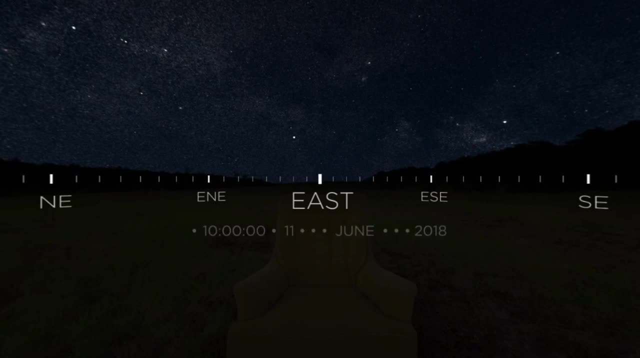 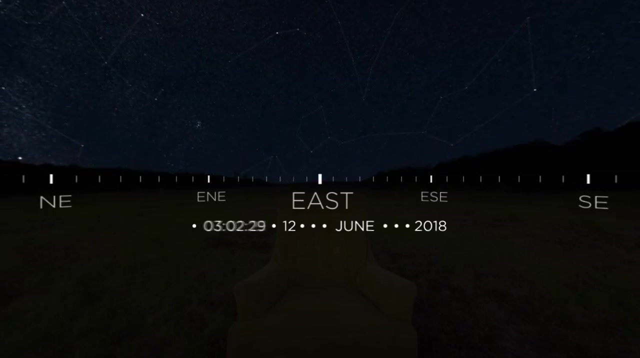 You'll run into the north star, Polaris. It's in the tail of a much fainter little bear, Ursa Minor. As the night passes, Polaris stays fixed in the north as all the other stars rotate around it. I should mention that the night sky will look different depending on where exactly you. 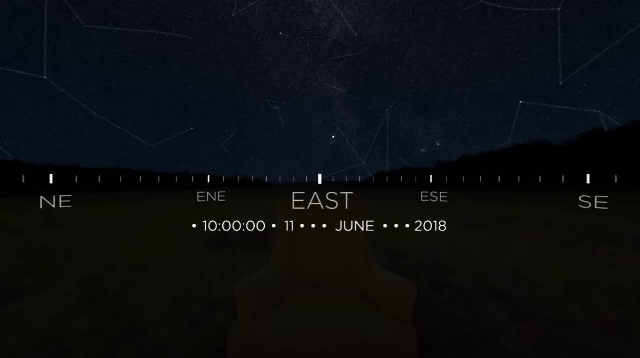 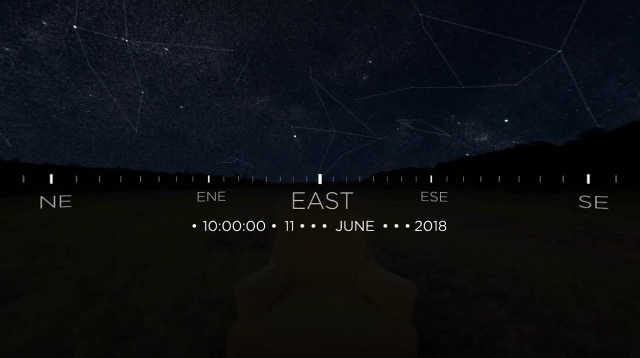 are At the North Pole, Polaris is directly over your head. As you travel south, Polaris moves lower and lower until at the equator it kisses the horizon. Here in Pennsylvania it's right in the middle. The sky also changes with the seasons. 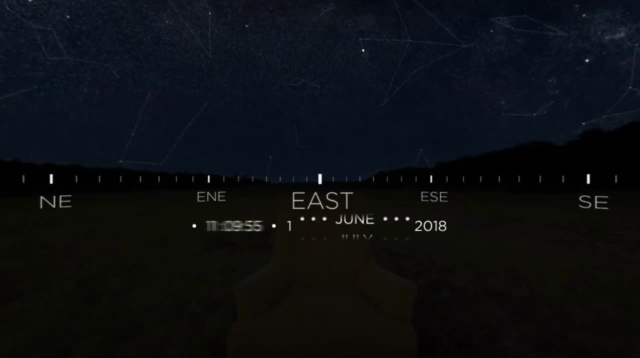 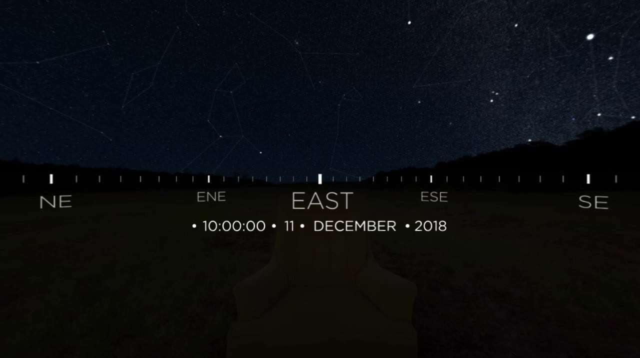 This is the sky now, 10pm on June 15th, But in a month the sky will look like this at 10pm, And by midwinter the 10pm sky will look very different, with a whole set of winter constellations. 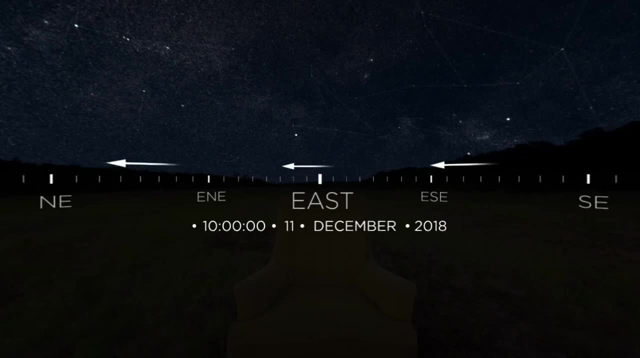 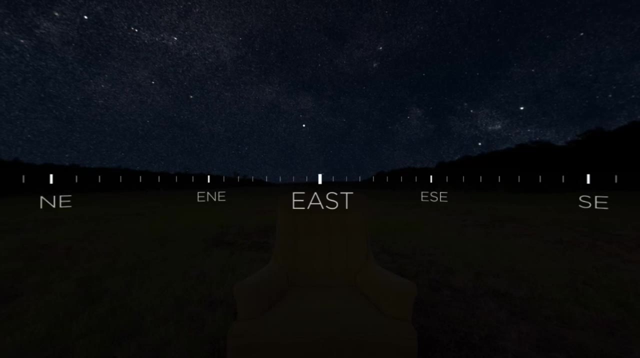 coming into view. But let's get back to summer and our guide, the Big Dipper. If we follow that same line from before, from those two stars at the Dipper's edge to Polaris, and then keep going about the same distance, again curving slightly, we'll reach Cassiopeia. 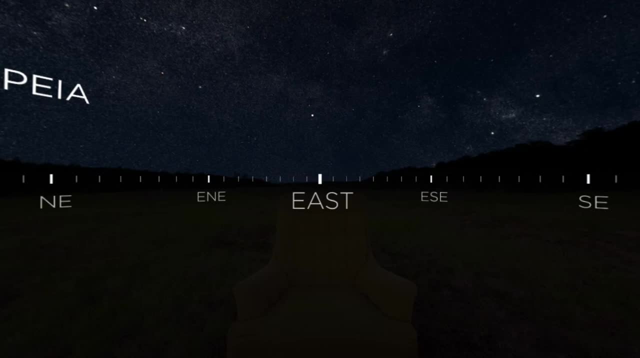 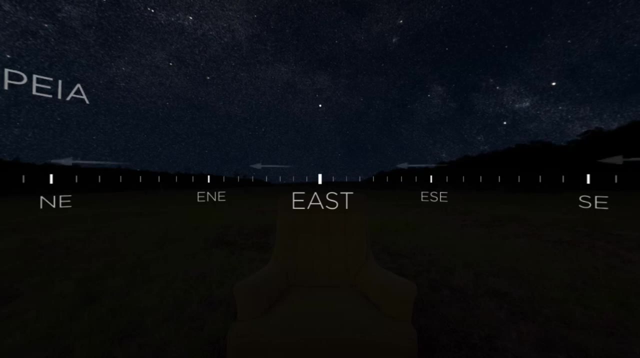 Look for a W in the stars. The ancient Greeks saw a vain North African queen on a throne- We'll be back in a minute- But people in northern Scandinavia and Siberia saw antlers. Okay, let's return to the Dipper. 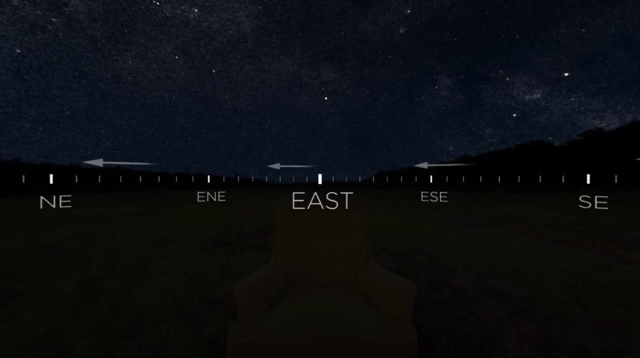 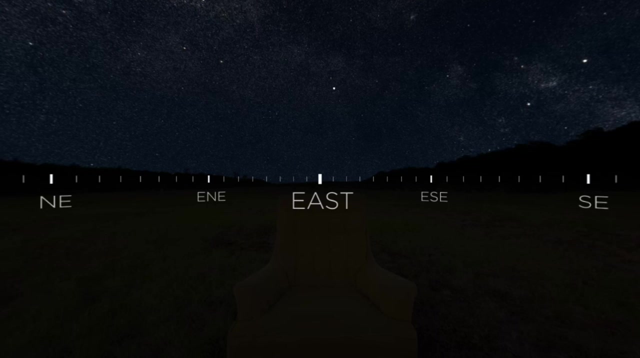 This time follow a line from the two other stars in the Dipper's bowl down towards the west until you hit a backwards question mark. This is Leo, a constellation that's been recognized as a lion for at least 6,000 years from ancient. 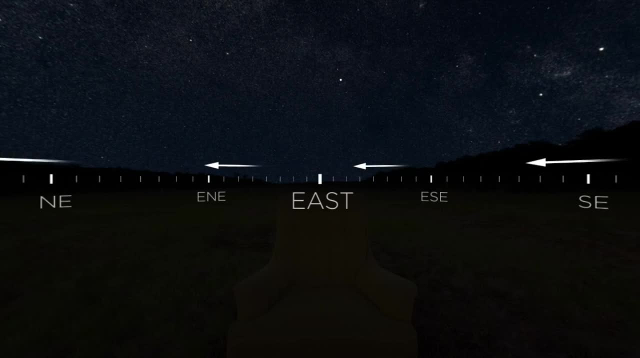 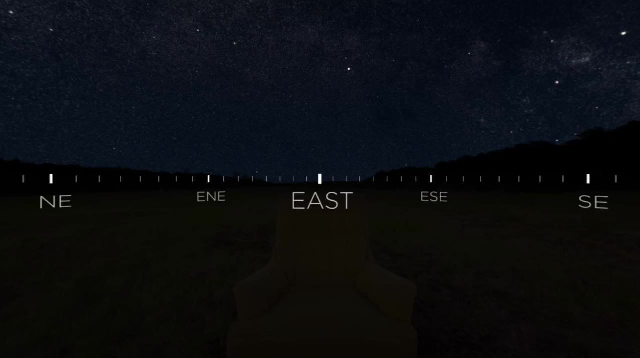 Turkey to ancient India, Back to the Dipper one last time. If you follow those same stars the other way, far across the sky to the east, you'll hit a bright star called Deneb. It's one of the most distant stars that you can still see clearly because it's so luminous. 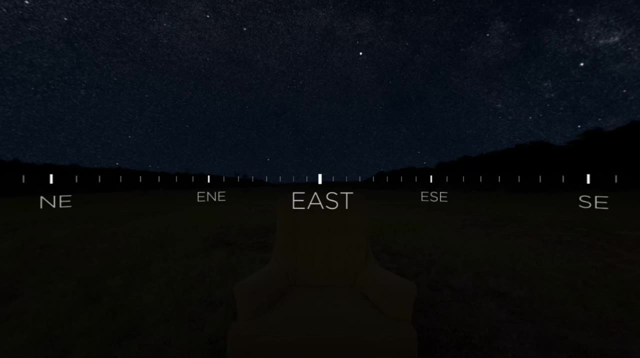 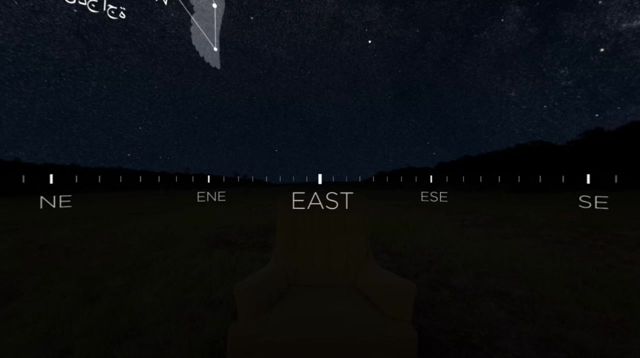 about 200,000 times brighter than our sun. Deneb comes from the Arabic for tail of the hen, and it is in a tail of a swan-like constellation called Cygnus. There are two more bright stars a little east of Cygnus. first by its left wing, Vega, in. 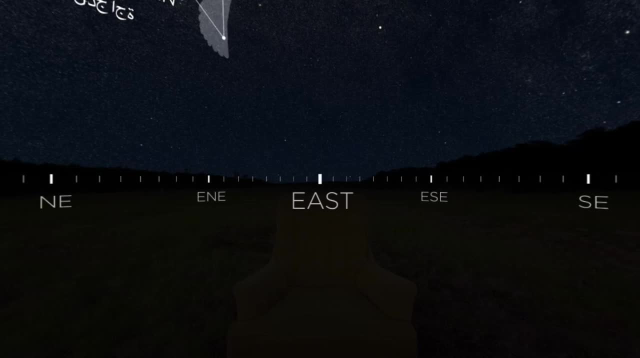 the constellation Lyra. Second. a little more towards the horizon you'll see Altair, the flying one. It's in Aquila, the eagle. These three bright stars are called the Summer Triangle. In China, Altair and Vega were seen as two lovers, a weaver and a cowherd. tragically, 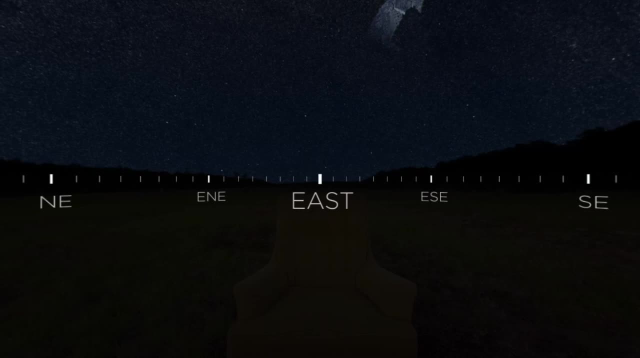 separated by the River of the Milky Way. As the night goes on, look south and you'll see a bright reddish star peeking over the horizon. This is Antares, in the constellation Scorpius. You can follow the line of its barbed tail, which looked like Maui's magical fishhook.